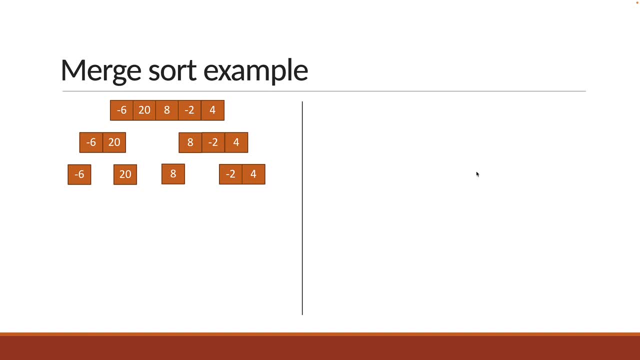 Now we again check for arrays which have more than one element and divide those, So the rightmost array will now split into minus 2 and 4.. At this point in time we have every element in the original array contained in its own. 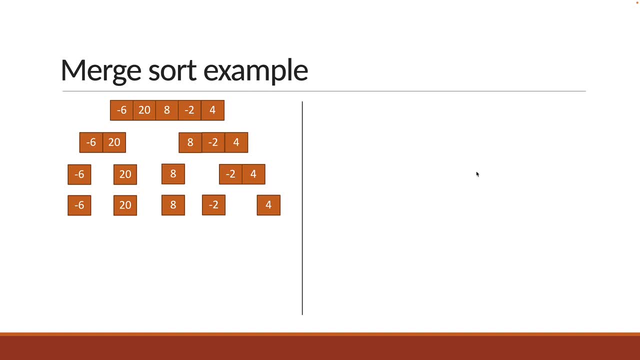 sub-array. Step 1 is complete. For step 2, we merge the individual sub-arrays into new sub-arrays, while ensuring the elements are sorted. Here is how it works: We take the two arrays and a temporary empty array to hold the elements as they are sorted. 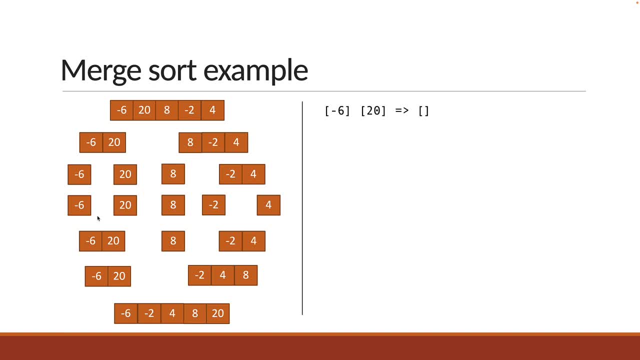 Let's start with minus 6 and 20.. Minus 6 is the left array and 20 is the right array. We check that the arrays are not empty. We then compare the first element in each array And push the smaller element into the temp array. 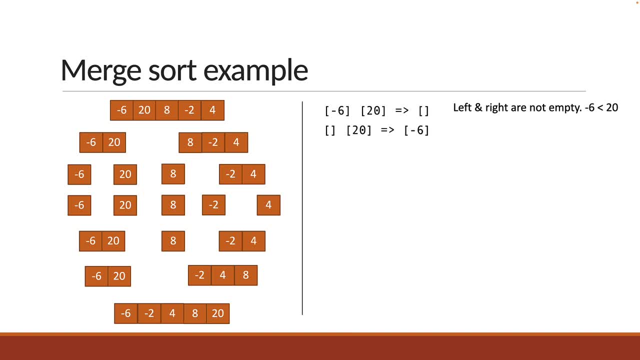 Here minus 6 is less than 20, so we remove it from the left array and push it into the temp array. Next we see that the left array is empty, So we simply push the element in the right array onto the temp array. 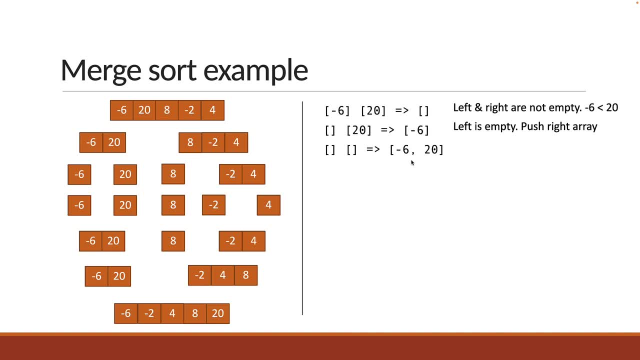 When both the left and right arrays are empty, we have the sorted sub-array, Step 2.. Let's repeat this process for 8 and minus 2 comma 4 to make sure we get this right. We have the left and right arrays. 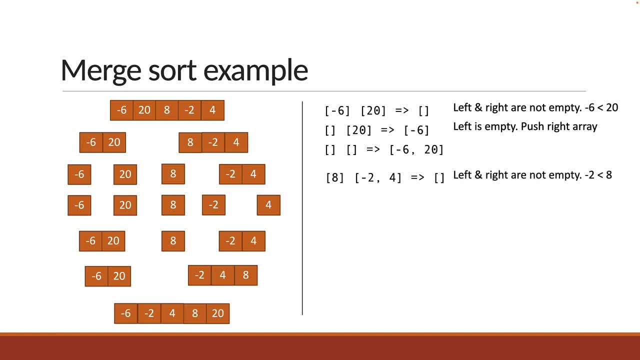 They are not empty. so we compare the first element in each array. Minus 2 is less than 8.. Push it onto the temp array. The left and right arrays are still not empty. So we compare the first element in each array one more time. 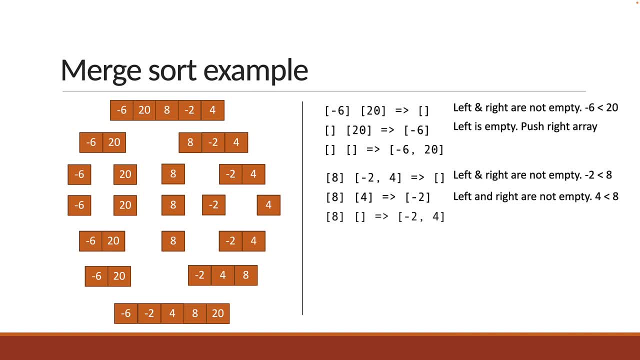 4 is less than 8.. So push 4 onto the temp array. Now the right array is empty. We simply push the left array onto the temp array. Both arrays are empty and we now have the sorted sub-array, Step 3.. 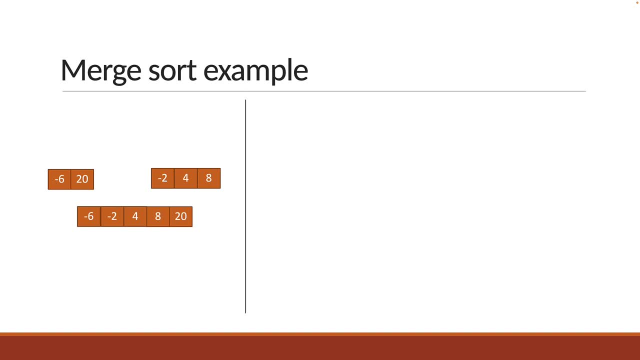 Let's repeat this process for 8 and minus 2 comma 4, to make sure we get this right, Step 4.. Let's repeat this process one more time for minus 6 comma 20 and minus 2 comma 4 comma 8.. 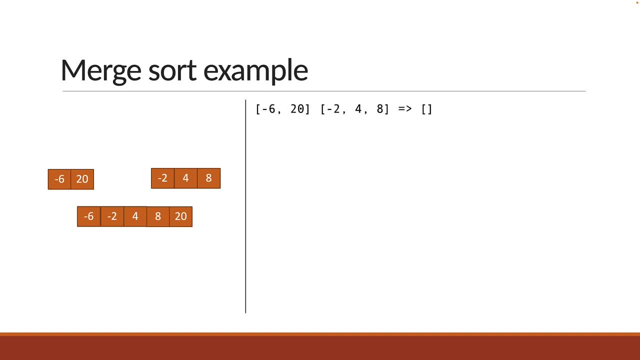 We have the left and right sub-arrays. Both are not empty. We compare the first element in each array. Minus 6 is less than minus 2.. Push minus 6 onto the temp array. Left and right are still not empty. 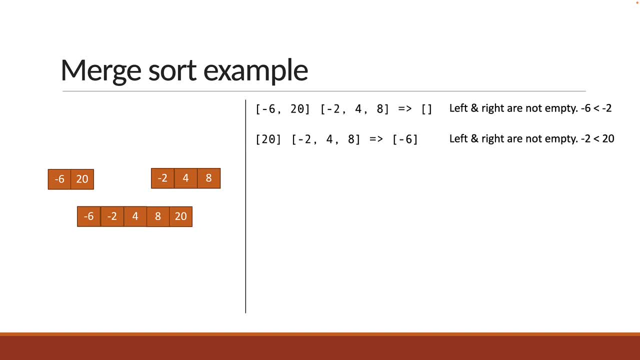 Compare the first element in each array. Minus 2 is less than 6.. So push minus 2 onto the temp array. The arrays are still not empty. Compare once again: 4 is less than 20.. So push 4 onto the temp array. 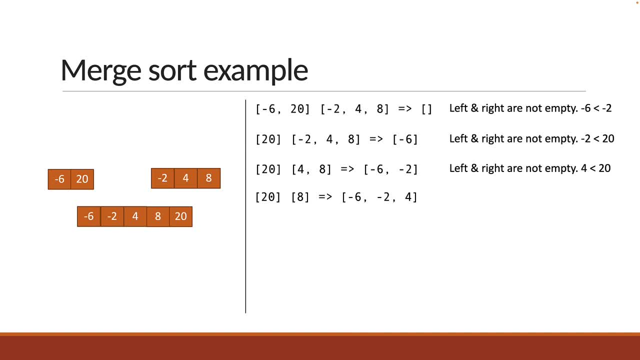 We still have an element each. So let's compare one last time. 8 is less than 20.. So push 8 onto the temp array. Now the right array is empty, So push the left array element onto the temp array. Both arrays are empty and we have just one sub-array left, which is the sorted array. 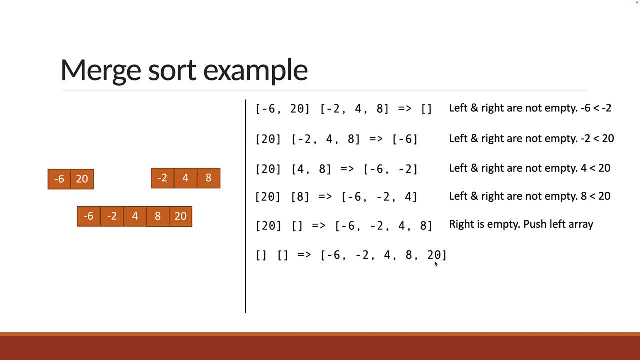 Minus 6, minus 2, 4,, 8 and 20.. This is how merge sort algorithm works. Alright, If you have understood the algorithm, Now is the time to pause the video. Pause and try implement the solution. 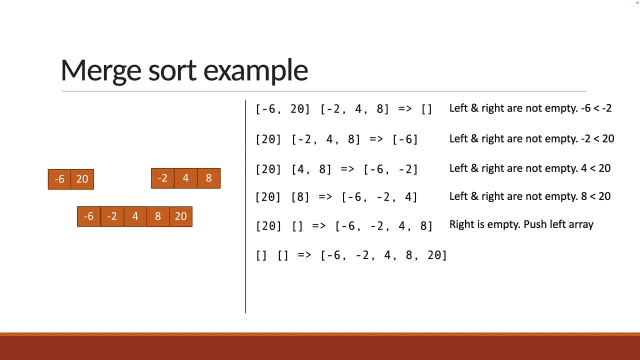 If you would like to solve together, let's do so in the next video.